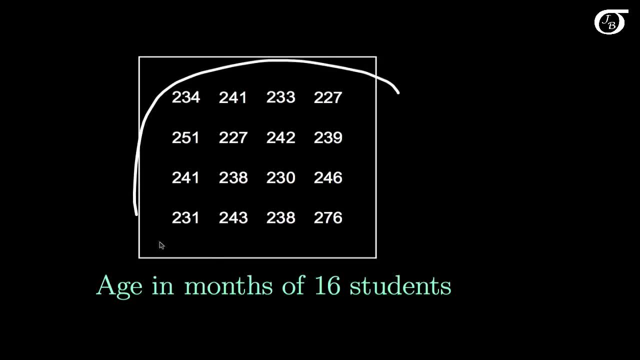 These are the true ages for the 16 students in the class And this is the reality of the situation. we can calculate the true population mean mu, and if we take the average of those 16 values, we would see that that is 239.8125.. 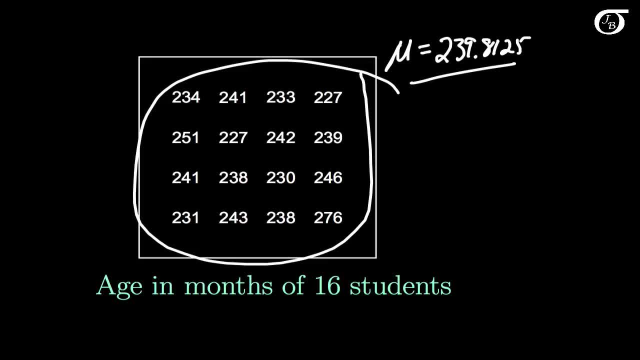 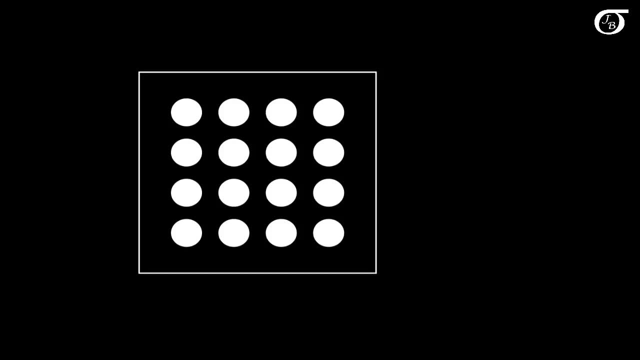 But that is an unknown value to the professor. To the professor, the reality of the situation looks something like this: There's 16 students with unknown ages. I'm going to number them so we can keep track of them. The professor is allowed to draw a random sample of three students and find out their ages. 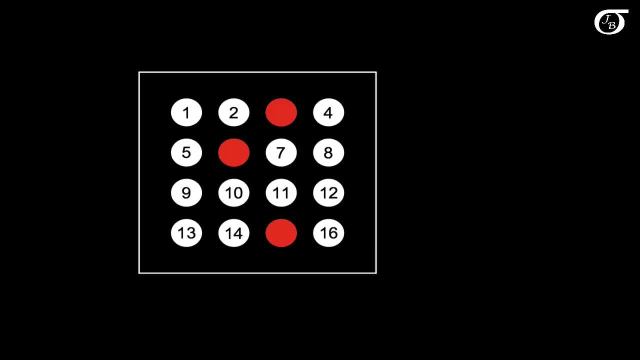 So let's randomly select three students. The red dots represent our randomly selected students and we can find out their ages in months. We get ages of 233,, 227, and 238.. And we could calculate the sample mean of those three values. 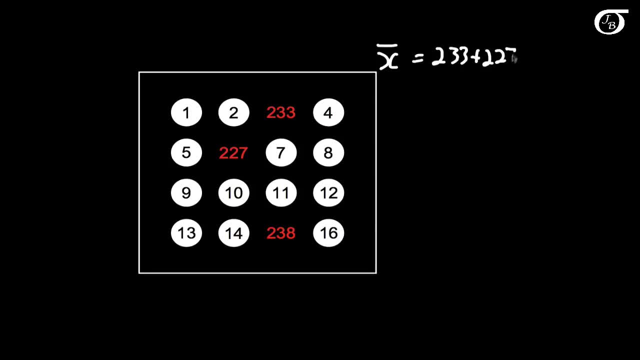 simply by adding up those values and dividing by 3. And we get a value of the sample mean of 232.67, when rounded to two decimal places. We're going to use this value of the sample mean to estimate mu, which is an unknown quantity to the professor. 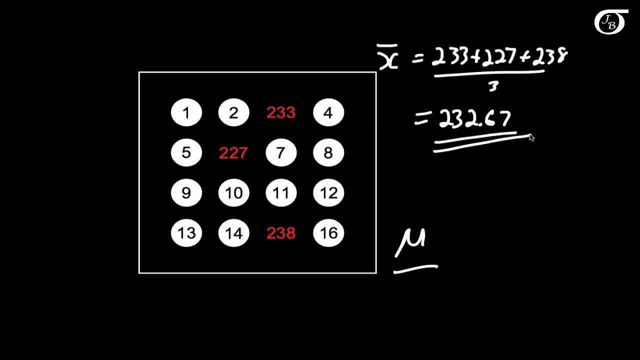 In addition to this single value, this point estimate that estimates mu. we would like to give some measure of the uncertainty associated with that value. How close is that value likely to be to the true value of mu? To answer that question, we use mathematical arguments based on the sampling distribution of X bar. 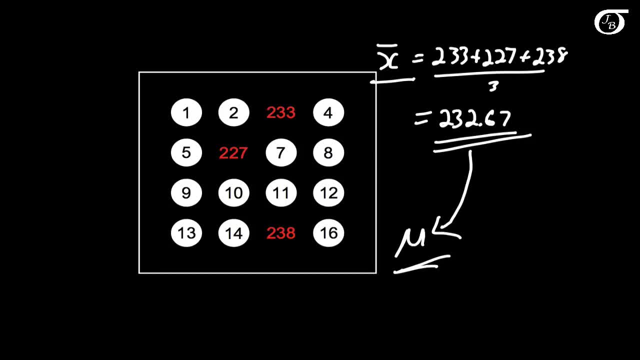 Related to that is the idea that if we were to draw another sample, we would be very, very unlikely to get this sample mean again. The sample mean is going to vary from sample to sample. Let's take a look at an example of that to illustrate. 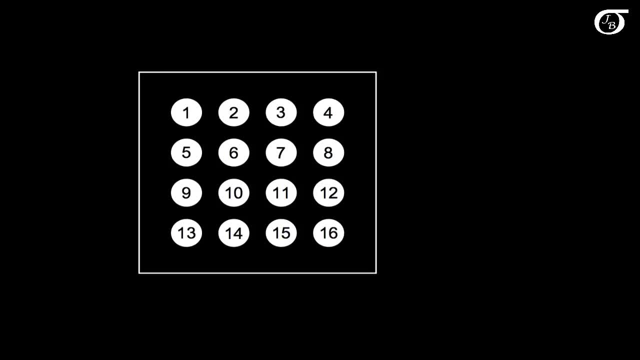 Here's our 16 students again and let's draw a random sample of size 3.. We get these three students and they have ages of 251, 238, and 276.. And we can again calculate the sample mean of those values. 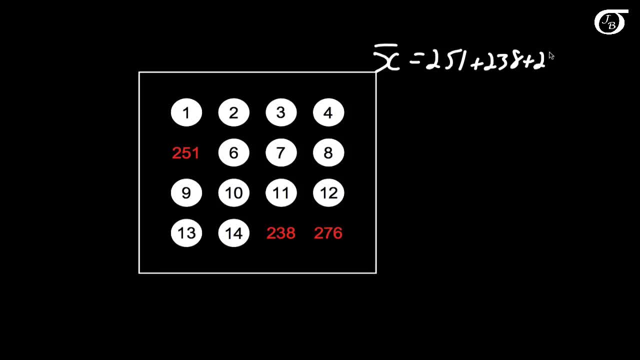 by simply adding them up and dividing by 3.. And this time we get a sample mean of 255.. And had we got this sample, we would use this value to estimate the unknown mu. Note that the sample mean we got here was different from the sample mean we got in our first sample. 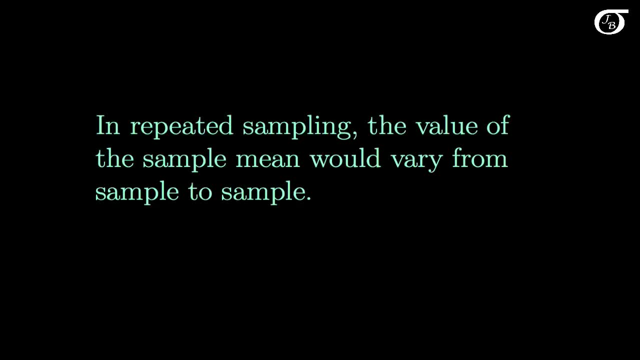 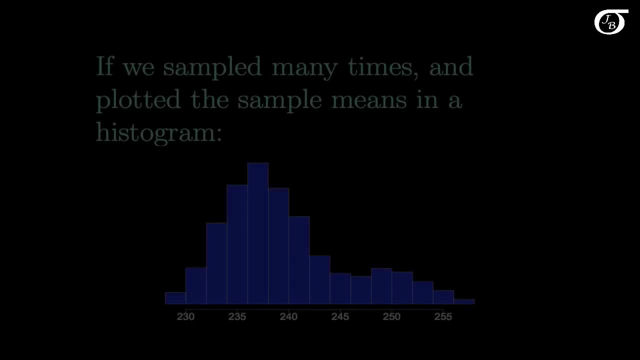 In repeated sampling the value of the sample mean would vary from sample to sample. The value of statistics vary from sample to sample. If we sampled many times, we did it twice here, but I've sped up the process using a computer and done it a million times. 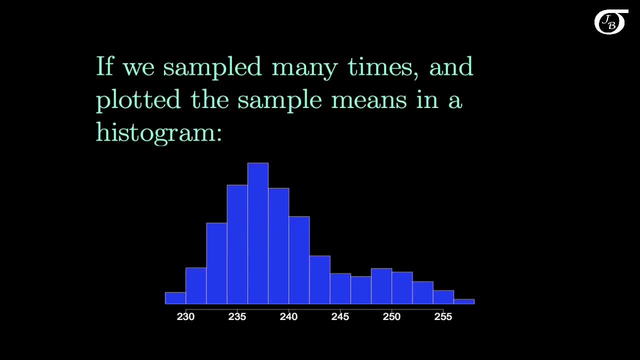 we plotted those sample means in a histogram. it would look something like this And because I've repeatedly sampled so many times, this histogram of sample means will very closely resemble the true sampling distribution of the sample mean. in this scenario, For a little perspective, I'm going to put in the population mean mu, with a red line. 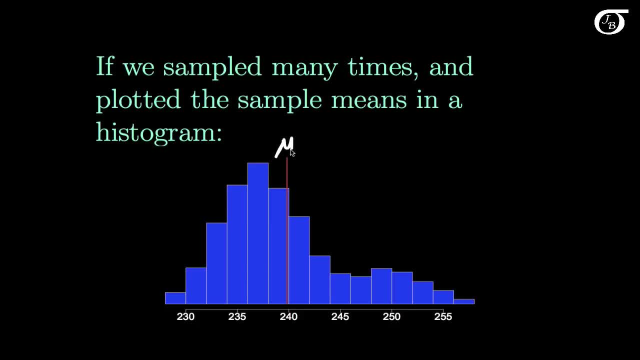 That's what this red line represents, our value of mu, which is about 240.. We can note that the sample mean will be distributed about the population mean in some way, As we'll learn later on. very often, the sample mean has a distribution that is approximately normal. 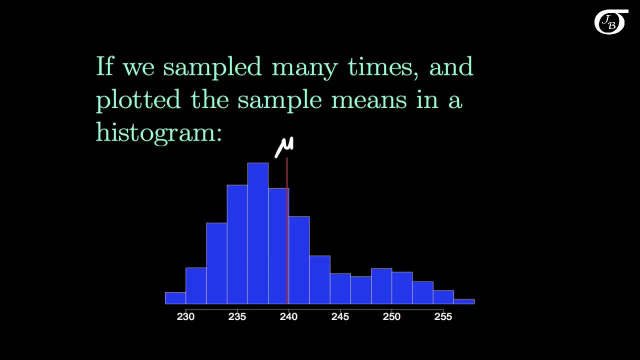 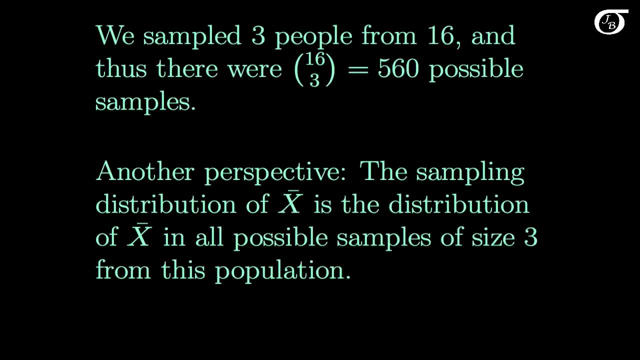 It doesn't look like that here, but in many situations the sample mean does have a distribution that is approximately normal. Here we sampled 3 people from 16, and thus there were 16 choose 3, or 560 possible samples. So another perspective on the sampling distribution here. 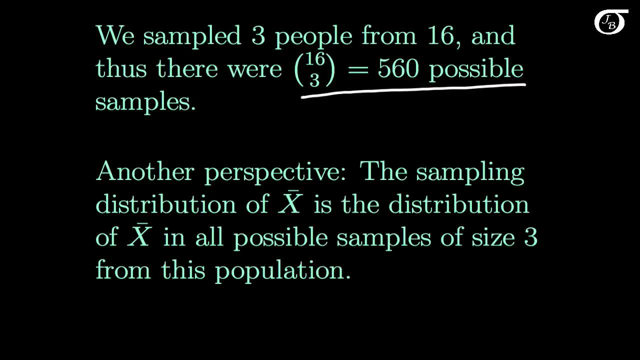 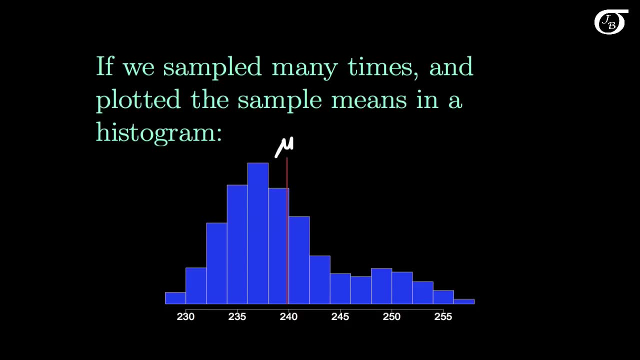 is that in this scenario the sampling distribution of the sample mean is the distribution of the sample mean in all possible samples of size 3 from this population. Going back to our histogram of sample means, we didn't have to actually repeatedly sample from the population. 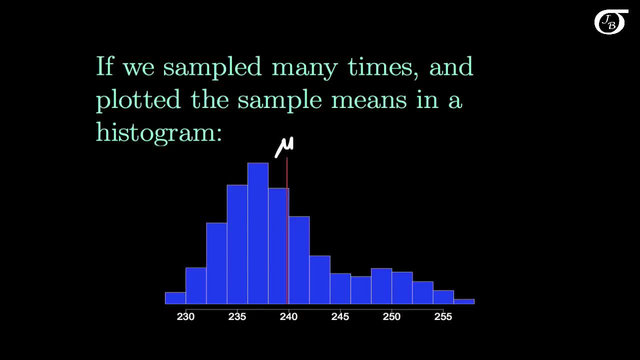 We had 560 possible samples, and so we could have worked out the exact sampling distribution of the sample mean in this scenario. But I wanted to illustrate the repeated sampling argument, And since we repeatedly sampled so many times, this histogram will very, very closely resemble.